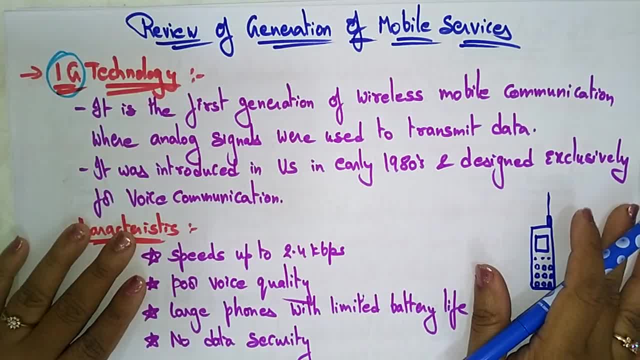 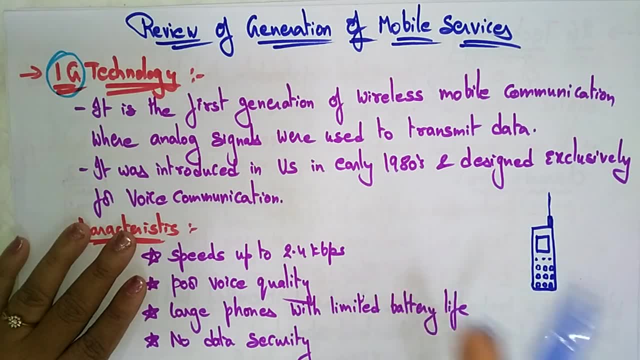 start with the technology 1g, first generation technology- in the view of mobile services. the mobile services, it's just: you can operate at whatever, at any time, at whatever the place you are. okay, so it is a movable, you can move from one place to another place. uh, you can operate that mobile. 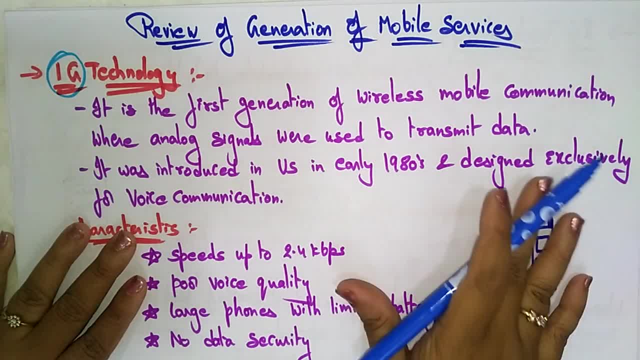 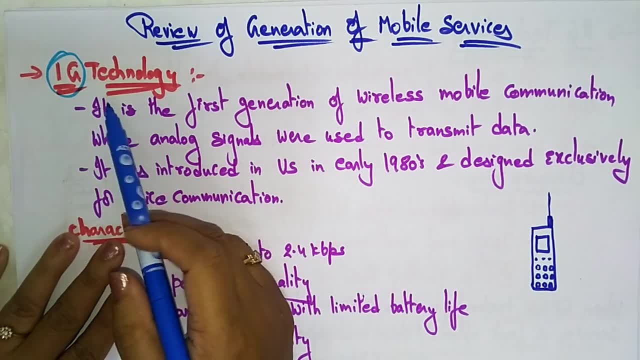 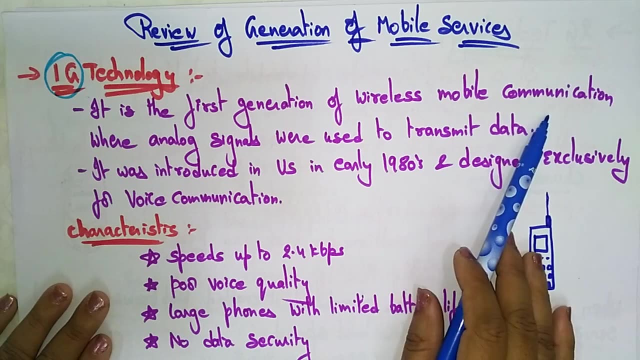 services. you can use that mobile services. so in that view of uh mobile services, what is the first starting generation? let's see: first technology is the 1g technology. that is the first generation. it is the first generation of wireless mobile communication where analog signals were used to transmit the data. so in the first, 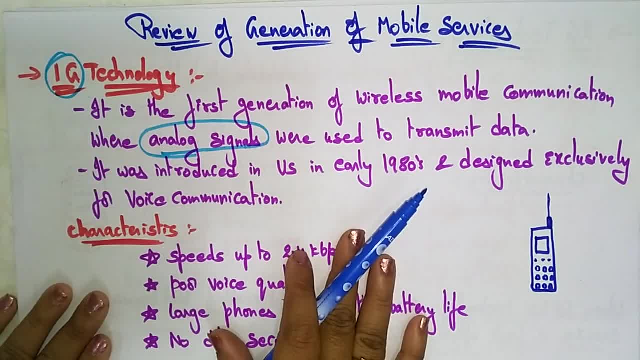 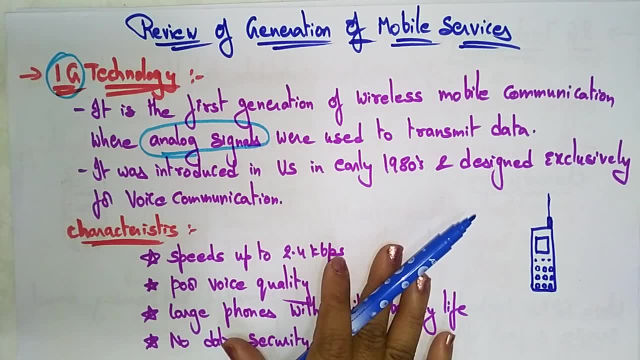 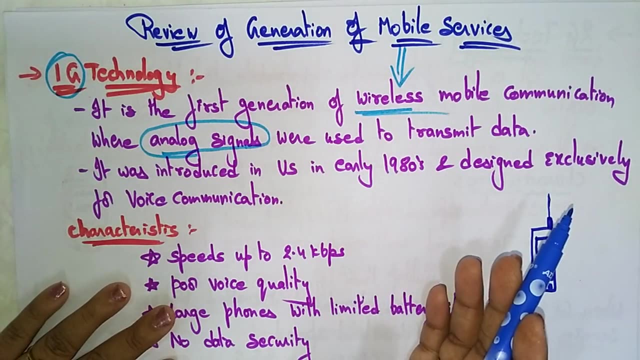 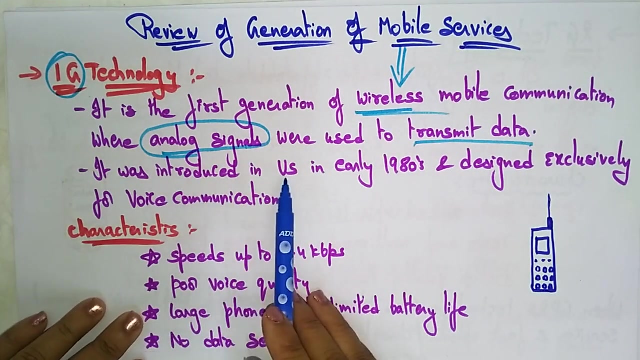 generation technology. okay, so, uh, we are using. we are using the analog signals, not the digital signals. the first for mobile wireless mobile communication. mobile means a wireless. okay, so in the first generation of wireless mobile communication we will use the analog signals, uh, user, to transmit the data. it was introduced in us in early 1980s. okay, the first. 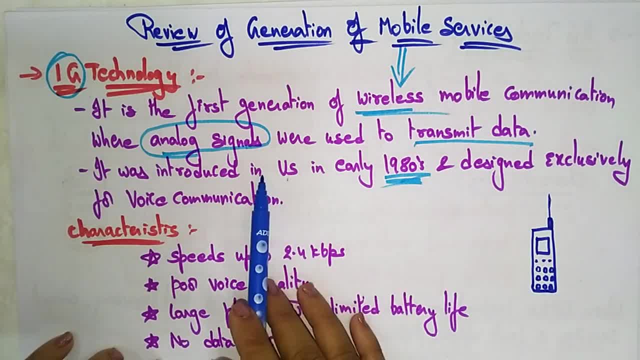 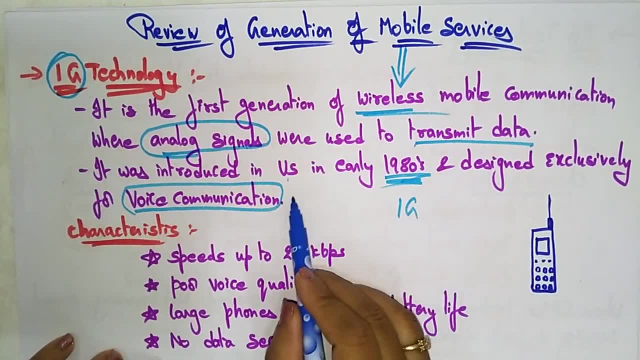 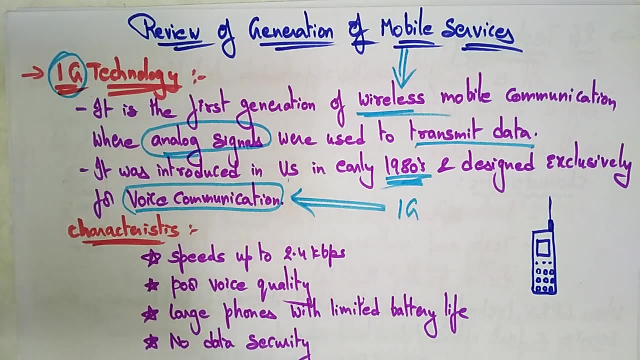 generation technology was introduced in the early 1980s in us and designed exclusively for voice communication. so the first generation, the 1g technology, will support only voice communication. okay, other than that, you can't- uh, you can't send the messages, you can't. 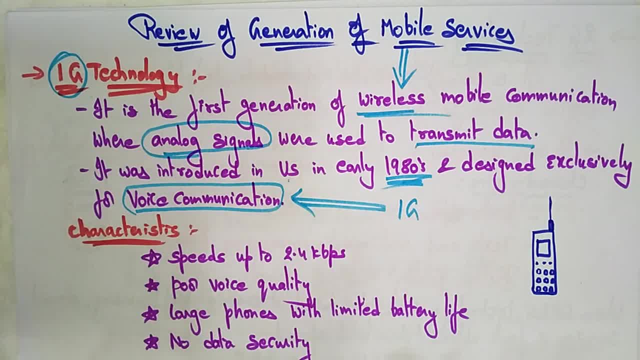 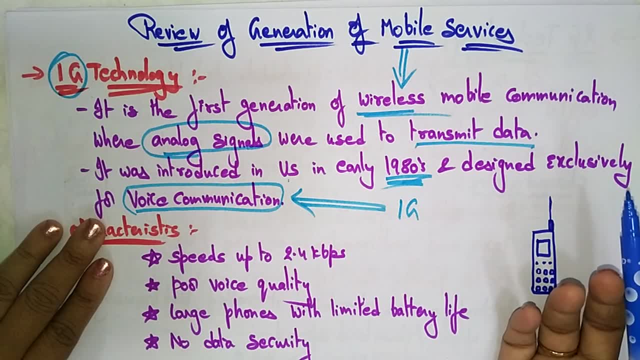 view the pictures? not at all. so in the 1g technology, in the mobile services, it is used only for the voice communication. then what is the difference between the graham bell, whatever the invented telephone- a telephone is also, uh used for voice communication- and the mobile service, the. 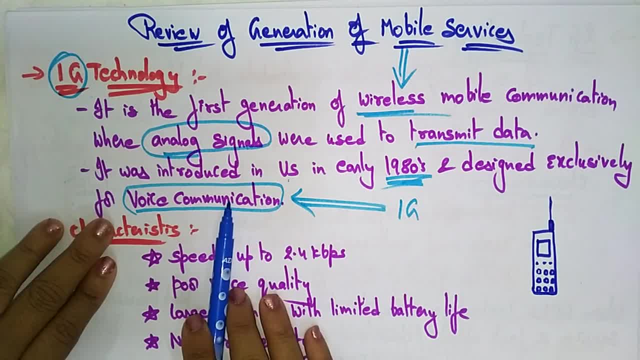 first generation technology is also used for the voice communication. the only difference between that telephone and the mobile services? the mobile services is a wireless mobile communication, whereas the telephone is a wired communication. the wire has to be connected and you can't move that telephone from one place to another place. 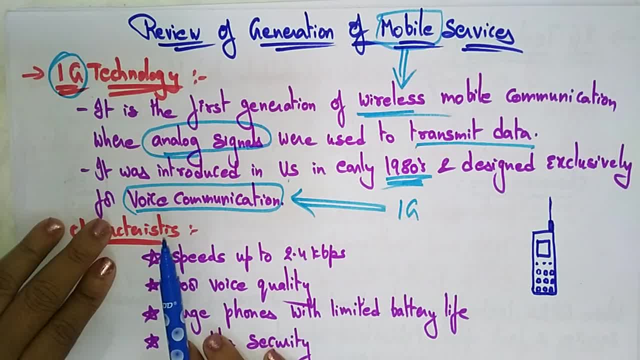 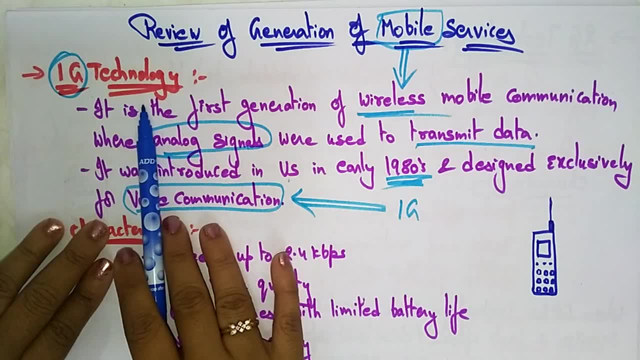 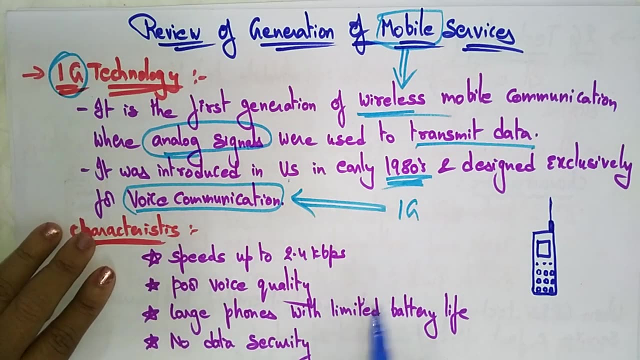 but you can carry the mobile, you can carry the mobile. so that is the only difference, uh, between the telephone and the mobile. and the first 1g technology, the first generation technology, uses exclusively for voice communication, so this will be look like this: it has a mobile phone like this: 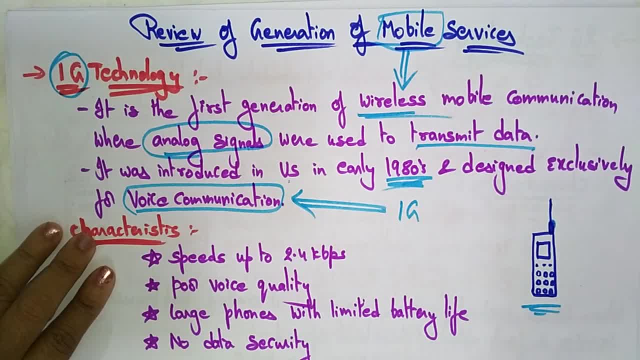 and there should be an antenna which is uh used to uh congress signals. okay, for the signal purposes, there is an antenna will be connected to this mobile. the characteristics of first generation technologies: the speed is up to 2.4 kilobits per second. only 2.4 kilobits per second. it is a poor. 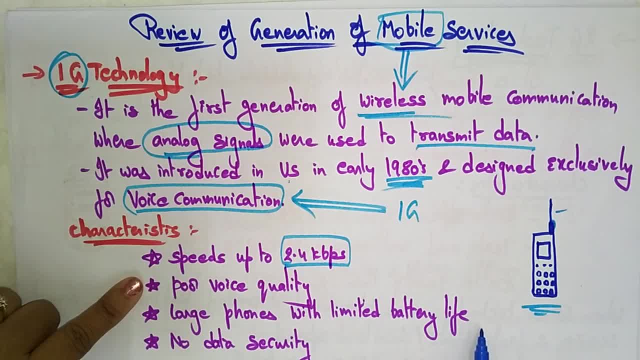 voice quality. large phones with limited battery life. the phones are very, uh, big in size, okay, so they are not portable means it is very big in size and the battery life is also limited. a small battery life will be there and no data security is there. this is a first generation technology of. 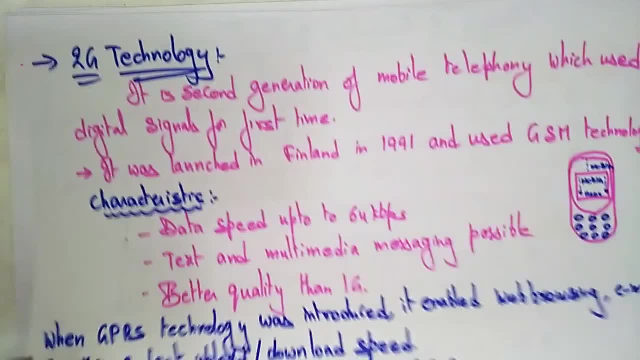 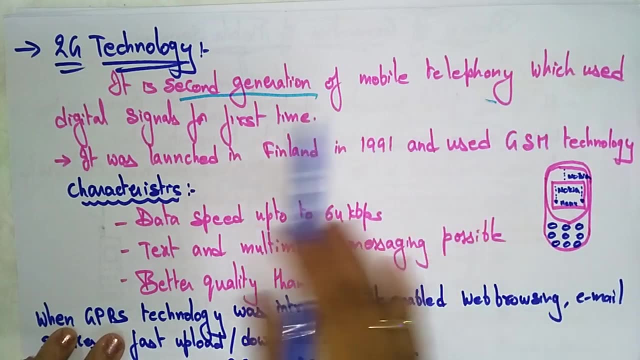 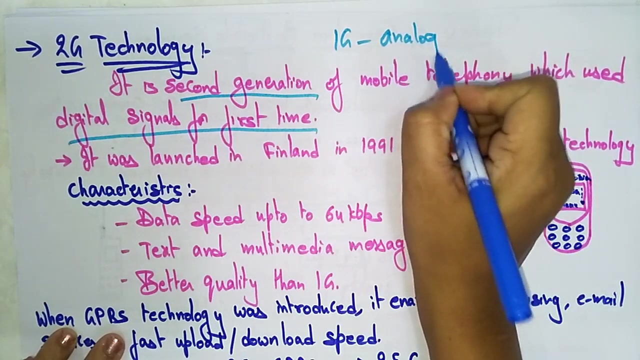 mobile services. now let's coming to the next generation, that is a 2g. so i hope you know that 2g technology. it is a second generation of mobile telephone which is using the digital signals first time, whereas in 1g we used only the analog signals. we used analog signals and whereas in the 2g, 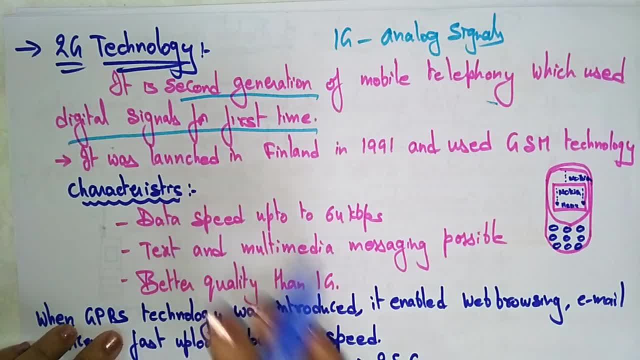 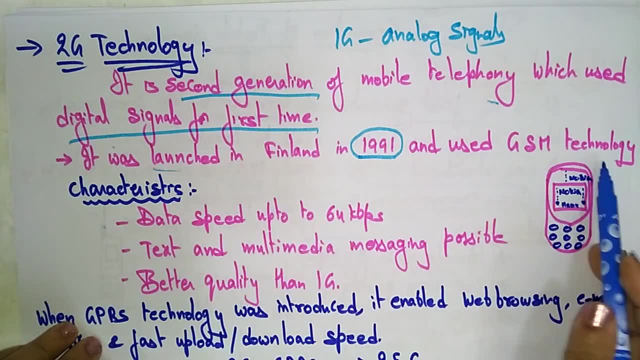 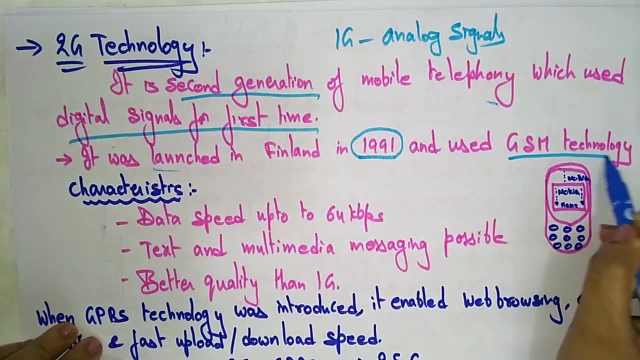 Second generation of mobile telephone uses the digital signals for the first time. It was launched in Finland in 1991.. It was started in 1991 and used GSM technology. Okay, The second generation mobile services use the GSM technology and it uses the digital signals and launched in Finland in 1991.. 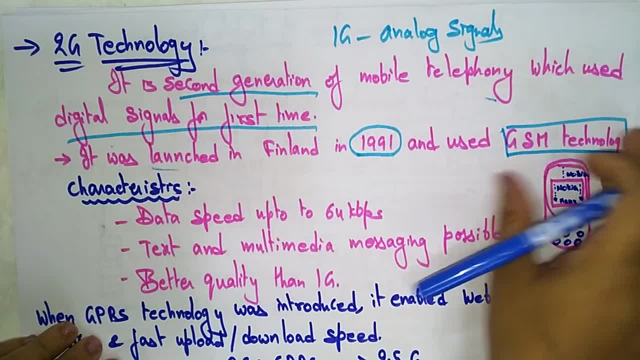 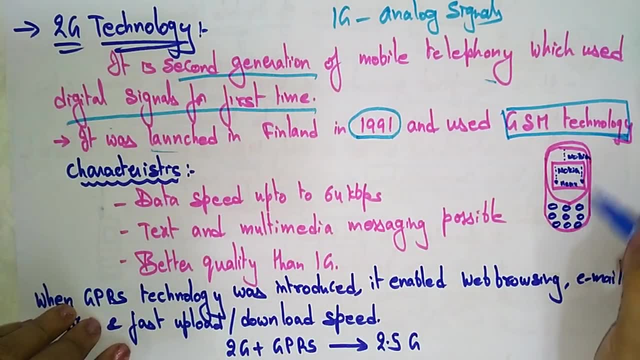 So remember these points. The GSM technology was introduced in the 2G technology, Second generation technology, So the mobile phones is like this: Previously the mobile phone, the Nokia mobile phones are look like this. They don't have antenna. like this: 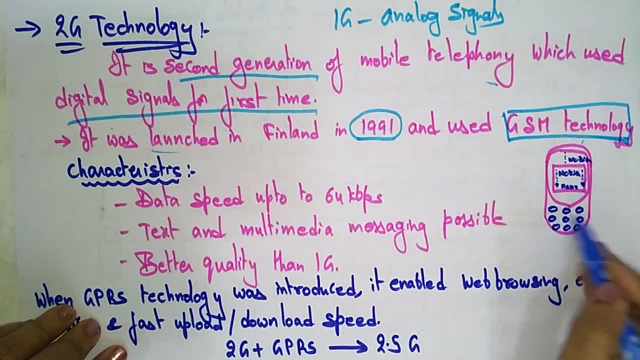 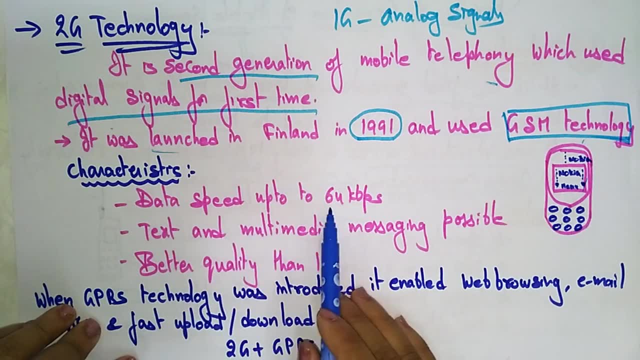 Only the screen will be there, and here the signals will be appeared and then dialing for numbers. That's it, Okay. The characteristics of the second generation technologies: the data speed is up to 64 kilobits per second, So previously in the 1G technology, you are having only 2.5 kilobits per second. 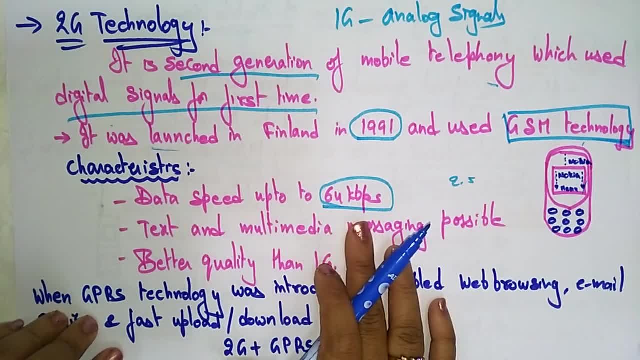 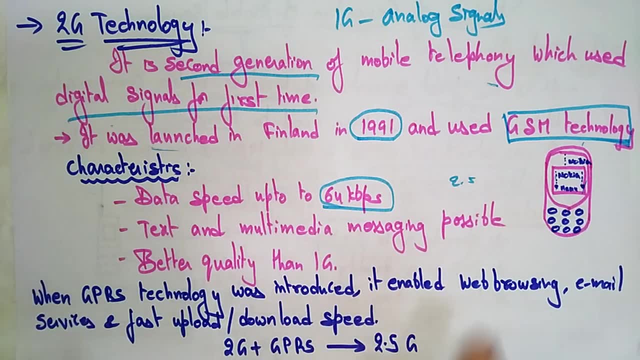 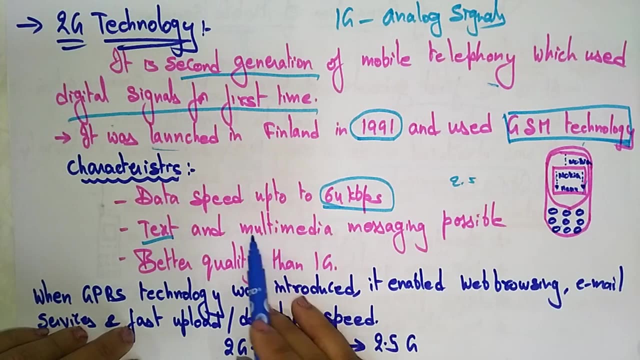 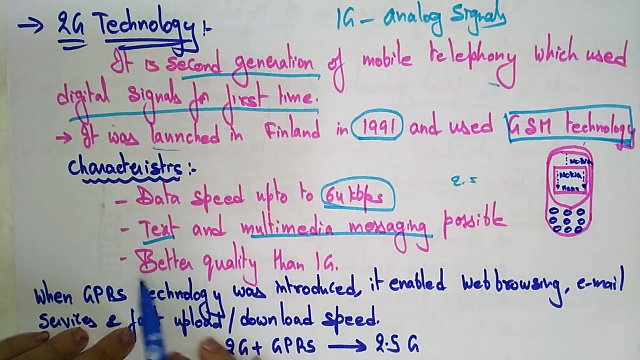 Whereas in second generation it is increased to 60. So the data speed is increased to 64 kilobits per second. The text and multimedia messages is possible. So whereas in 1G technology only it is used for the voice communication, But in the 2G technology you can able to type the text and the multimedia messages also you can send a data transfer can be either text or multimedia messages and the better quality than 1G. 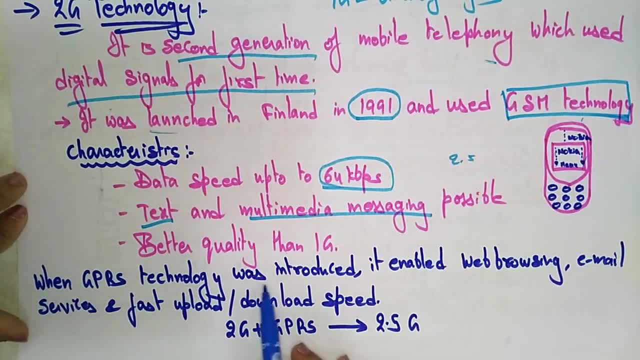 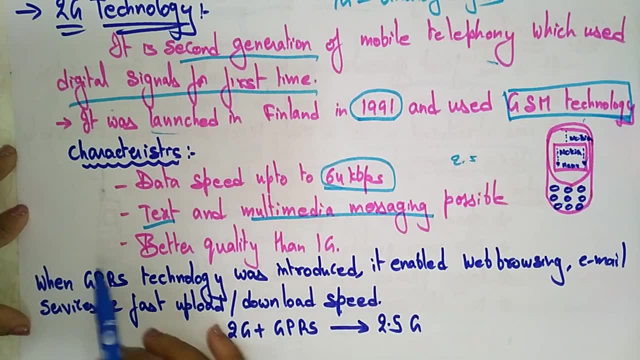 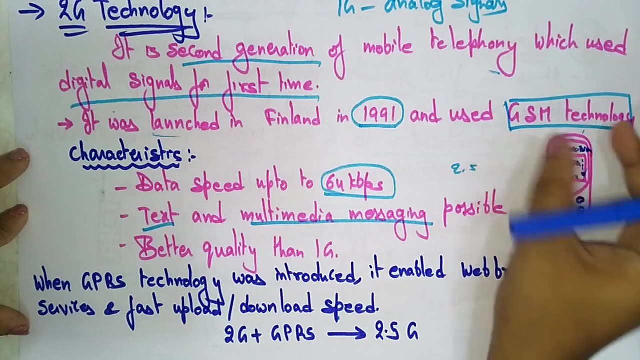 Okay When GPRS technology was introduced. it enables the web browsing. It enables the web browsing, email services and fast upload or download speeds. So already 2G technology is having the GSM technology, Even though the GSM technology- after the GSM, they added the GPRS technology, also GPRS technology. 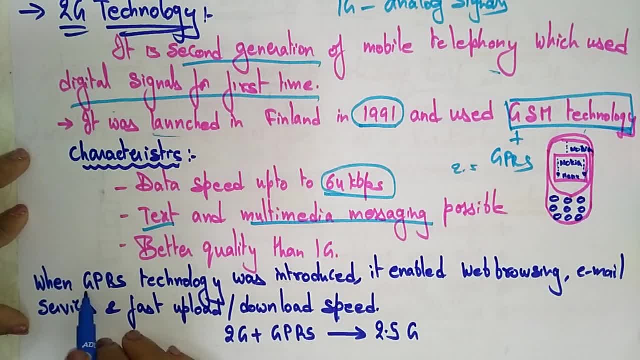 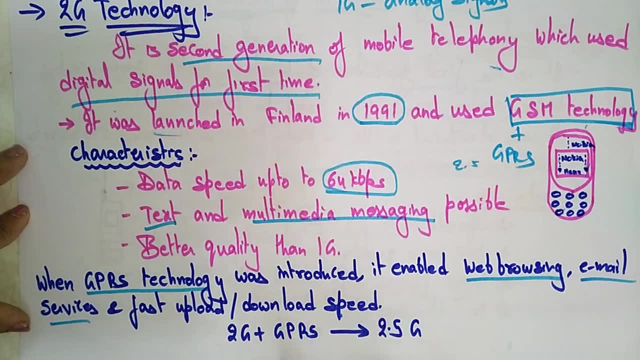 If the GPRS technology was introduced, then this is going to enable the web browsing. You are able to browse the mails and you can open the mails and you can upload a download. So the speed will becomes the speed when- whenever the GPRS technology was introduced. 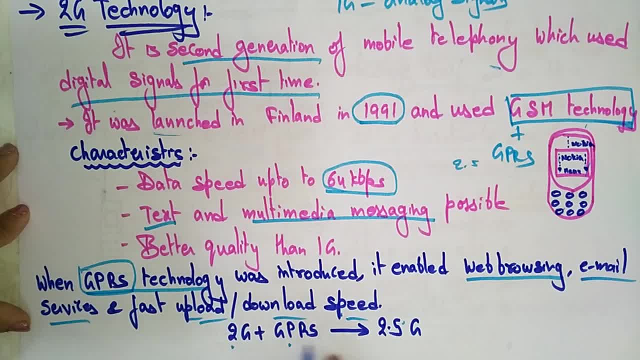 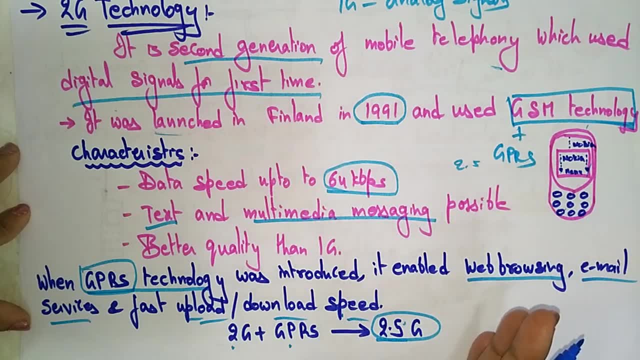 Okay, So the 2G along with GPRS technology is a 2.5 generation. You call it as a 2.5 generation technology. A 2G technology is advanced by adding the GPRS technology, which is enabled the web browsing and the email services and the uploads and the downloads fast. 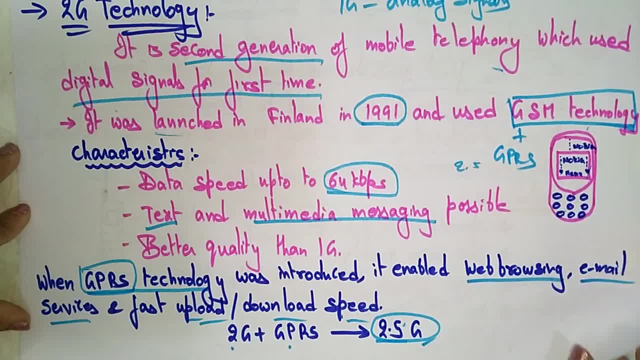 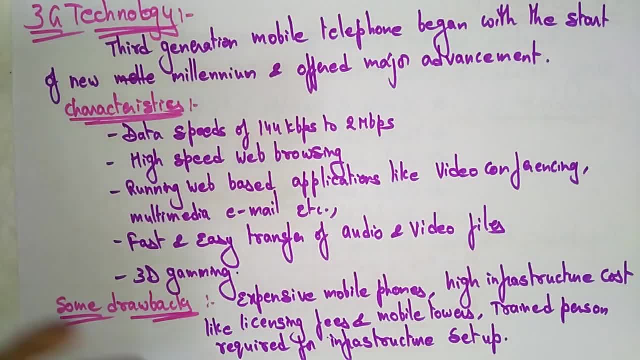 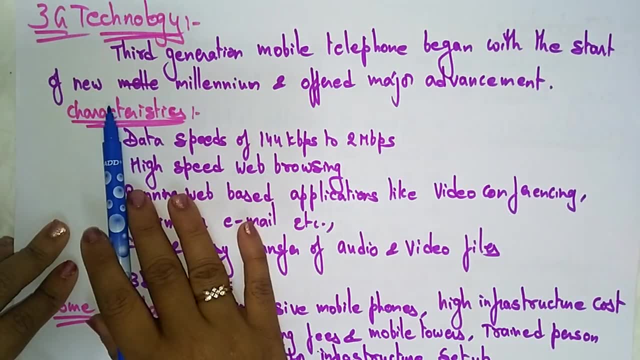 That type of technology you call it as a 2.5. Now coming to the next generation in the mobile surveys, that is a 3G technology. The third generation mobile telephone begins with the start of the new millennium and offer the major advantages. 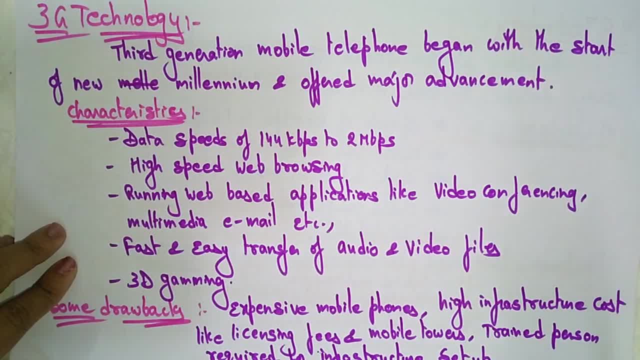 So the 3G technology is offering the major advantages when compared to the 2G. The characteristics: the data speed is from 144 kilobits per second to 2 megabits per second. Okay. Whereas in the 2G, 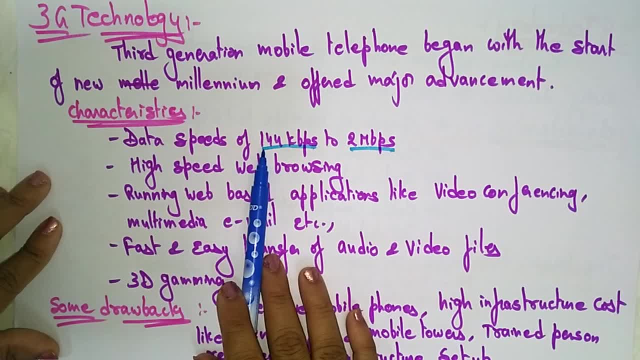 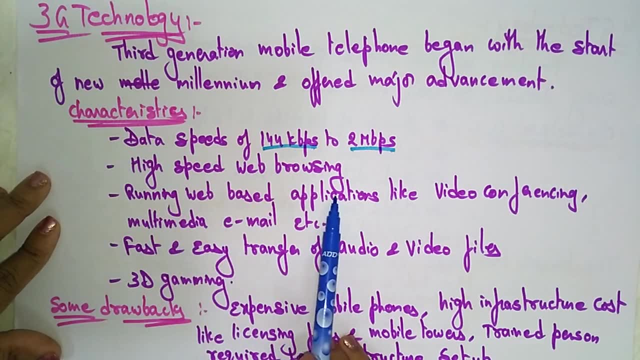 is having only 64 kilobits per second, but here it is increased between 144 to 2 megabits per second. high speed web browsing, running web applications like video conferencing, multimedia email- everything will be started when we are using the 3g technology. a video conference is added. 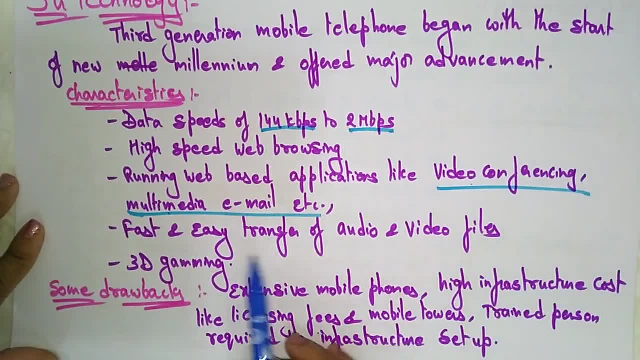 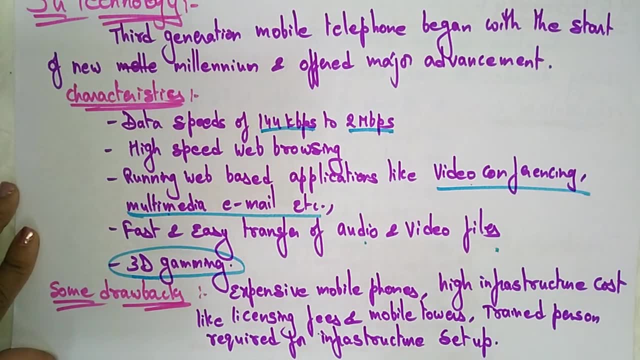 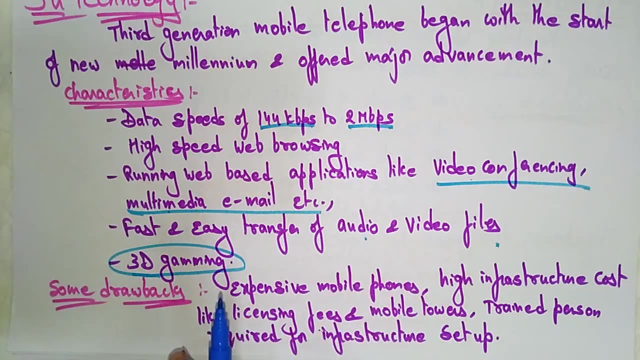 advantages to this 3g technology: fast and easy transfer of audio and video files and your 3d gaming is also supporting in the 3g 3d third generation technology. sorry, but even though it is having all the features and it is offering the major advantages, it is having some drawbacks. 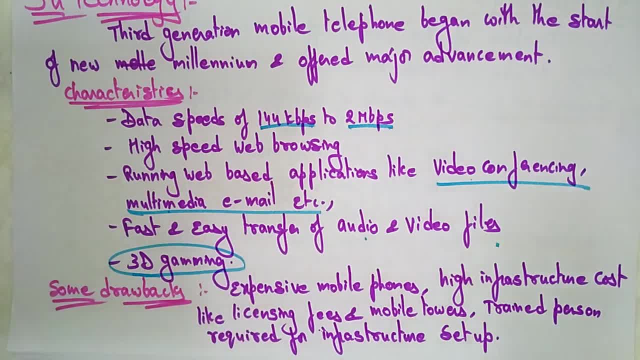 so, because of those drawbacks where they are introduced, latest advanced to the 3g. what are the drawbacks here? here, the expensive mobile phones, high infrastructure costs like licensing fees, mobile towers, trained persons required for infrastructure setup- everything will be required for 3g technology. okay, the, whatever the. 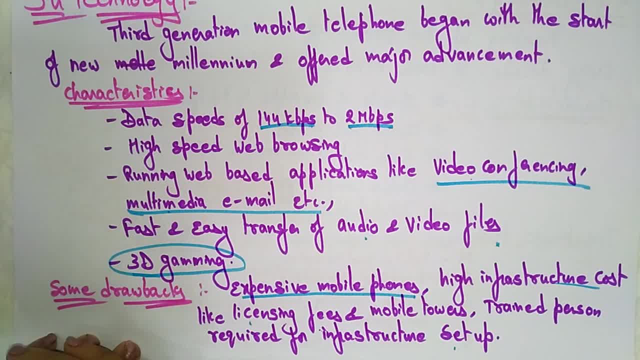 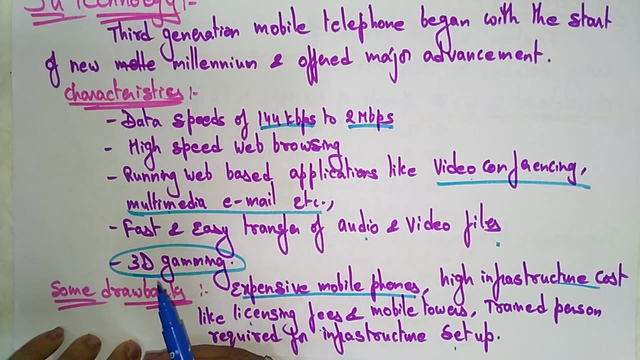 mobile phones that you wanted to purchase and that should support the 3d. 3g technology means the mobile phones are expensive. infrastructure is cost. why it is in infrastructure is. cost of infrastructure is high because of licensing. whatever your uh want to be installed, okay, a. 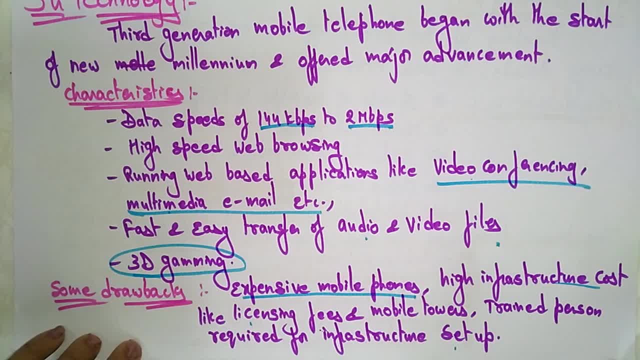 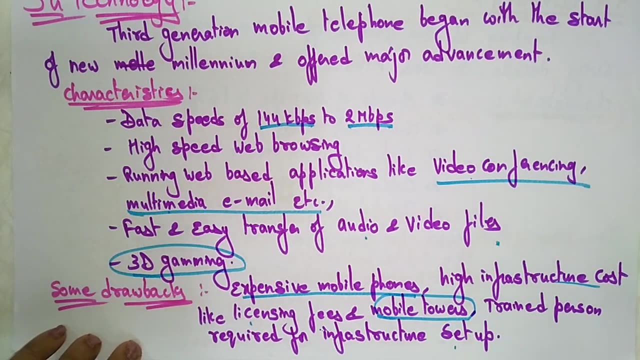 licensing fee should be there and the mobile towers has to be introduced in each and every place so that the 3g technology can be uh available to the people. okay, so without the towers you can't get the 3g signals. if the mobile towers are present, uh in each and every area, you will receive the 3g. 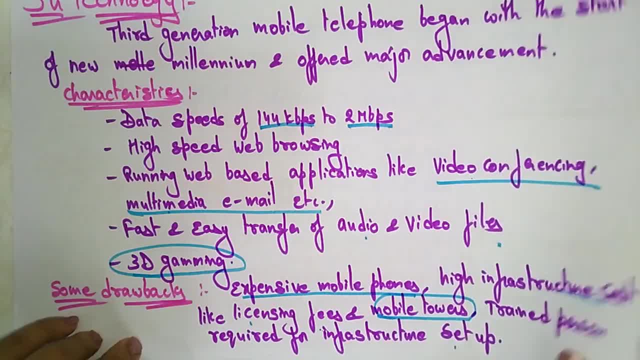 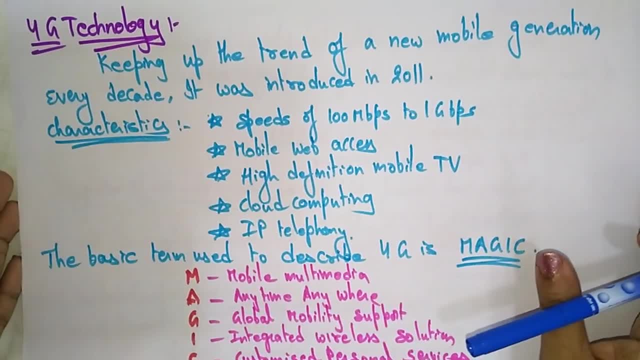 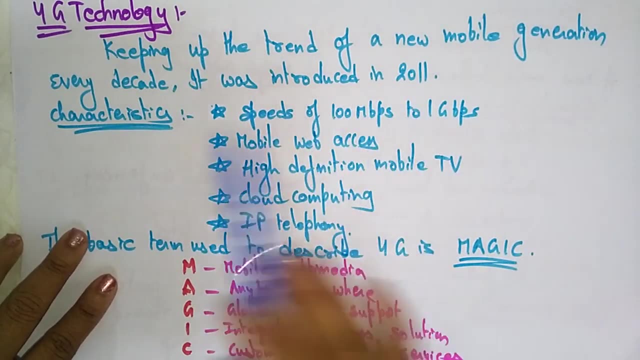 signals. trained person required for infrastructure setup. okay, so now let's come into the next generation, that is, a 4g technology, the fourth generation technology, keeping up the trend of a new mobile generation. every decade, a new mobile technology will be introduced every decade, every decade, decade. it was introduced in uh, every decade. okay, so it was introduced in 2011. what are the? 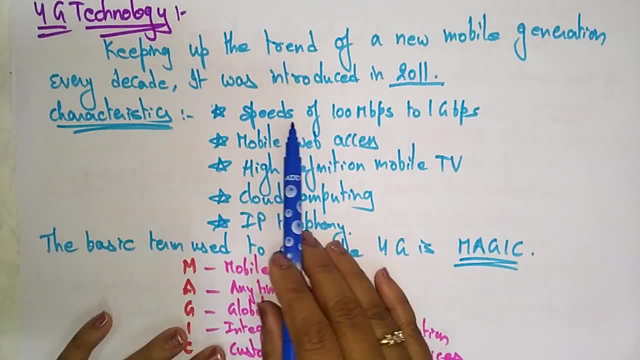 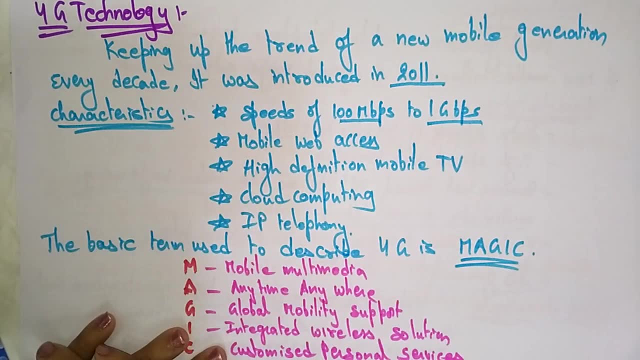 characteristics of this fourth generation technology. the speed is increased from 100 megabits per seconds to 1 gigabits per second. i think everyone nowadays using the 4g technology only mobile web access will be there. high definition mobile tv will be. you can connect to that cloud computing. 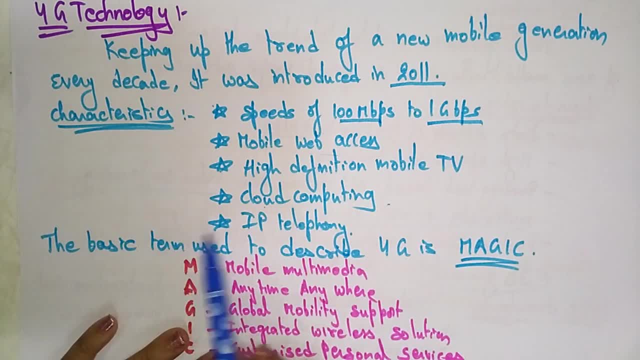 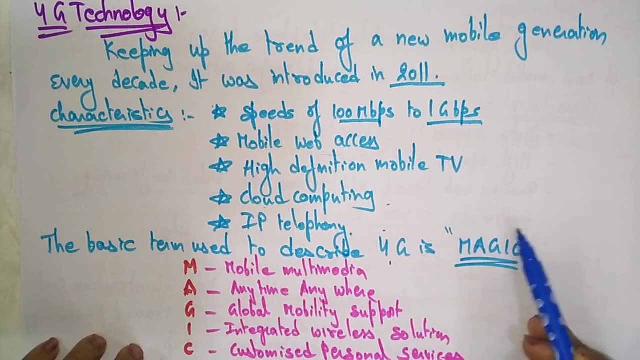 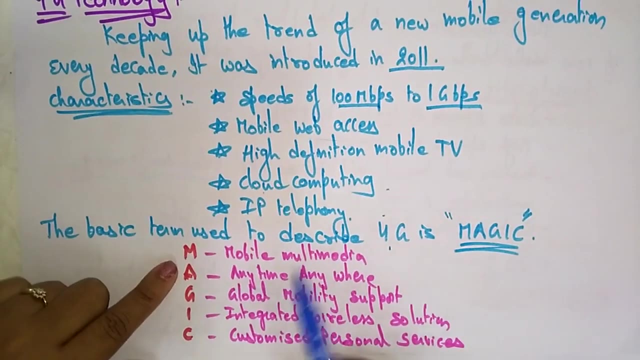 facility will be provided in the 4th generation technology. ip telephony will be there. the basic term used to describe the 4g is: we call it as a magic and simple words. we call the fourth generation technology as a magic. n means mobile multimedia, a means anytime, anywhere, g means global. 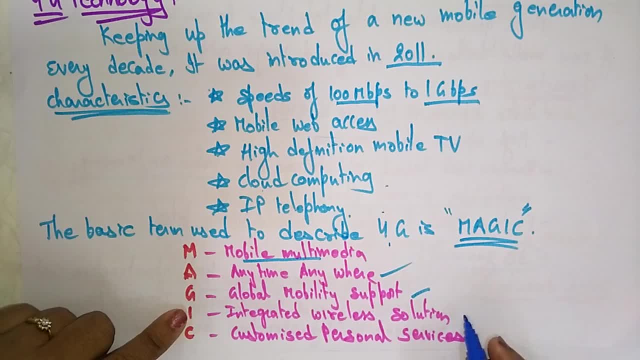 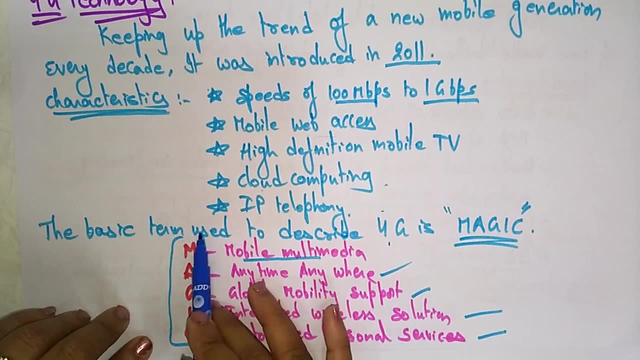 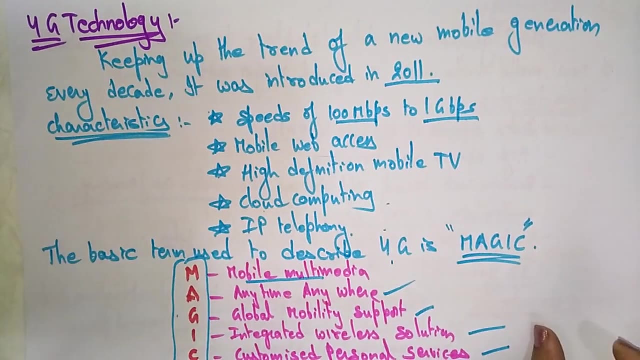 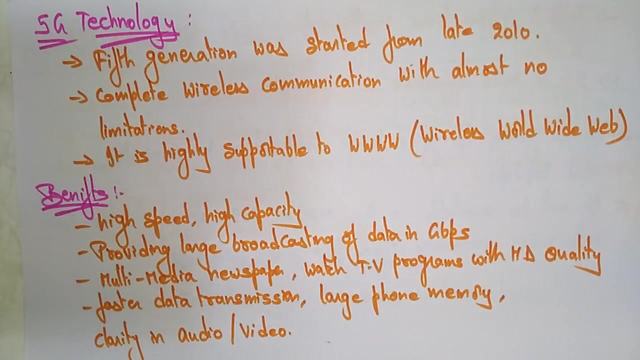 mobility support. i. integrated wireless solution. c- customized personal services. okay, so that's why this fourth generation technology is having all these features. that's why we call it as a magic. okay, so nowadays everyone is using this fourth generation technology and fifth generation technology is also introduced. okay, but not, uh, very much. at present we are not. 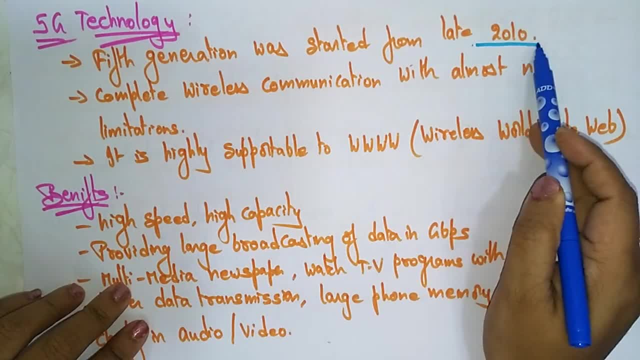 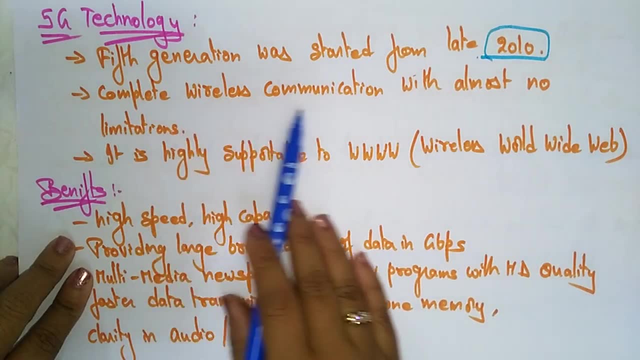 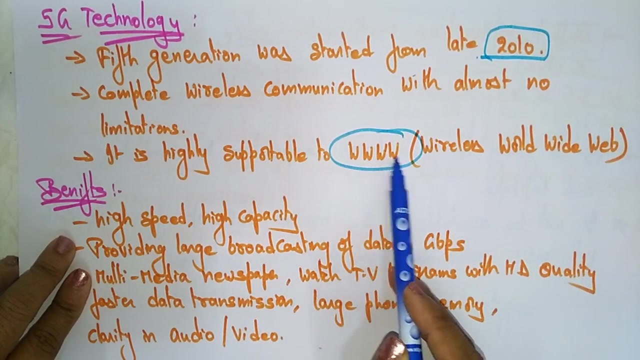 using that. the fifth generation was started from late 2010. only, okay, we already, they are already started. the fifth generation technology, it is a complete wireless communication with almost no limitations. with almost no limitation. it is highly supported to www. that is a wireless world wide web. it is going to support wireless world wide web. 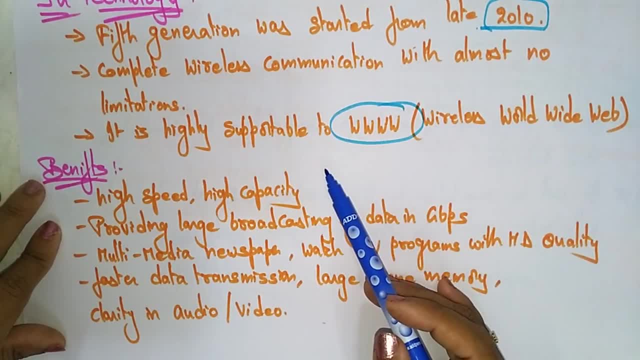 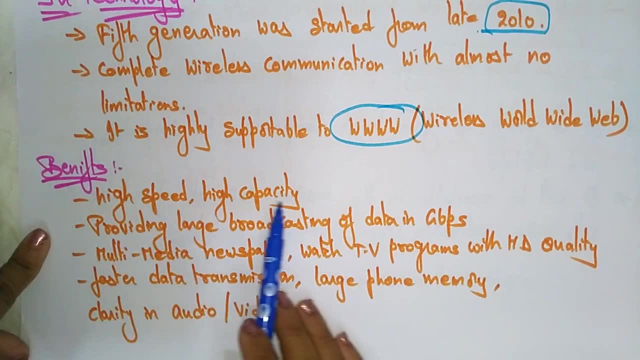 means the fourth generation technology is supportable to this uh. not only the world wide web, it's a wireless world wide web. the fifth generation technology benefits are high speed, high capacity, providing large broadcasting of data in gigabits per second: multimedia newspapers, watch tv programs with hd qualities. 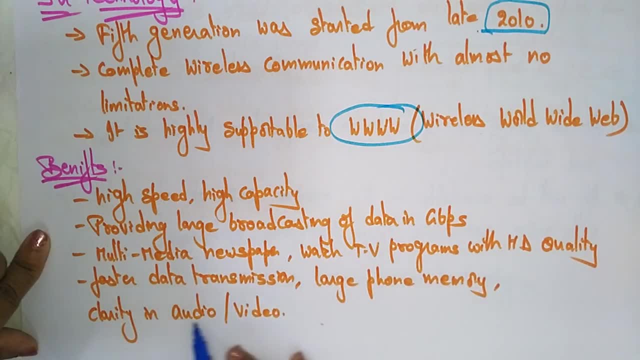 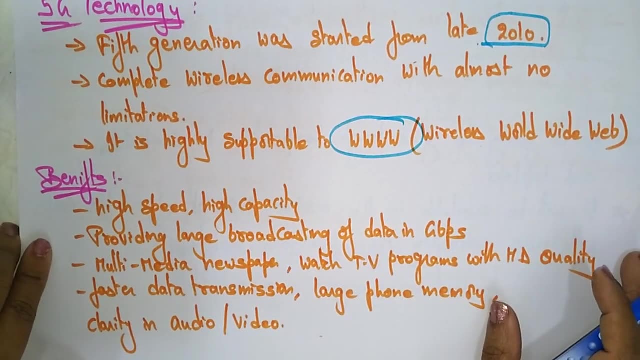 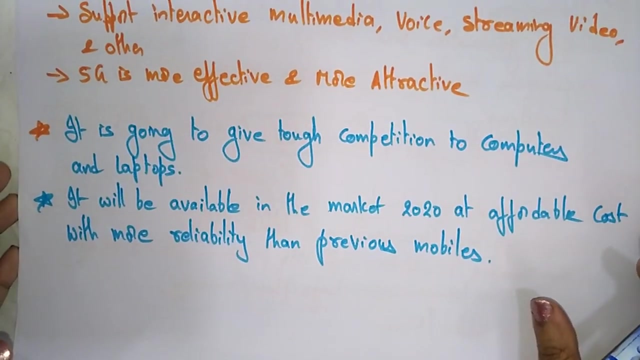 faster data transmission, large phone memory, clarity in audio or video. so all the high end features will be provided in the fifth generation technology. okay, so it's a complete wireless communication with almost no limitations. it supports the interactive multimedia, voice, streaming videos and other. the fifth generation is more effective and more. 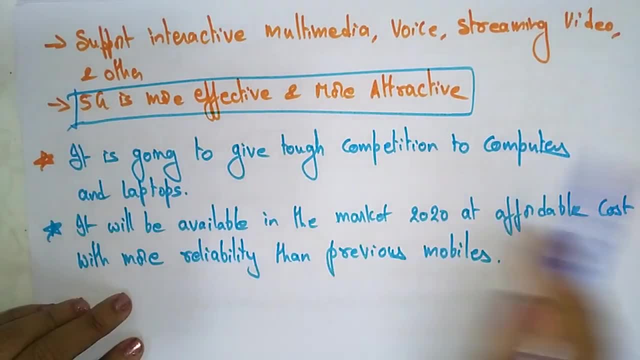 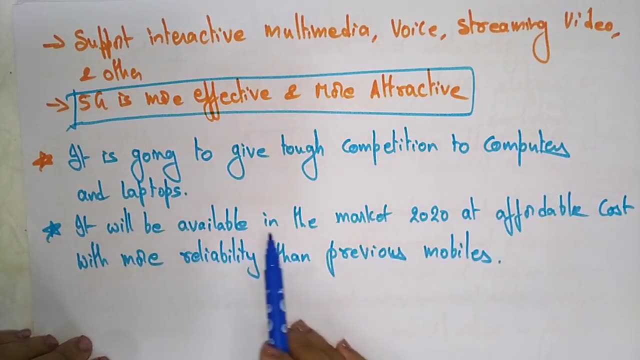 attractive. it is more effective and more attractive. it is going to give tough competition to computers and laptops, but it will be available in the market at 2020 at affordable cost with more reliability than previous mobiles. actually, now it is available, but it is uh, having a more expensive. 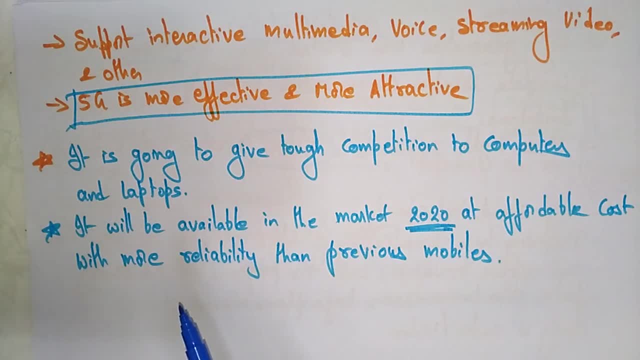 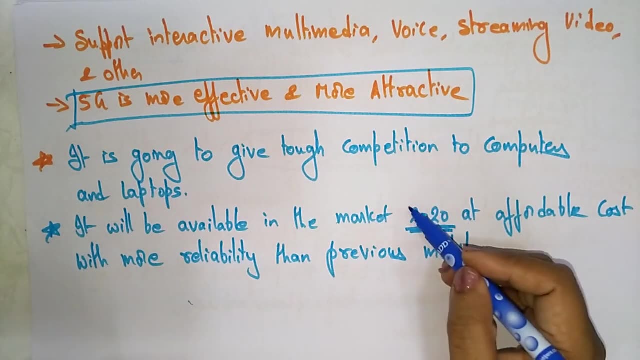 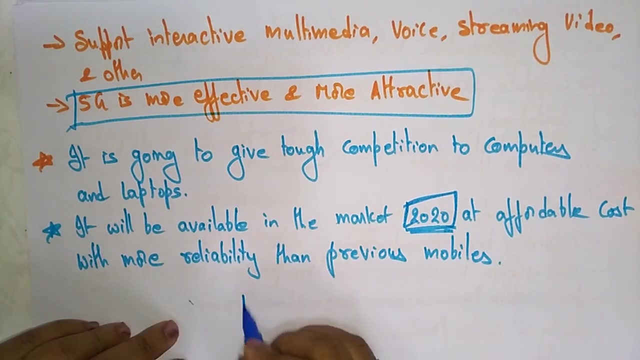 so they are trying to make uh affordable cost with more reliability than the previous models, and they will- mostly they will- release in the market in 2020, hope so. okay, so these are the different generations of the mobile services: 1g, 2g, 3g, 4g. so we are using in the 4g and next, 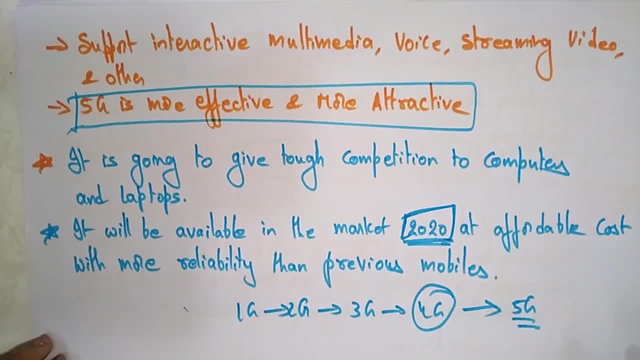 generation will be the 5g, fifth generation technology. thank you.